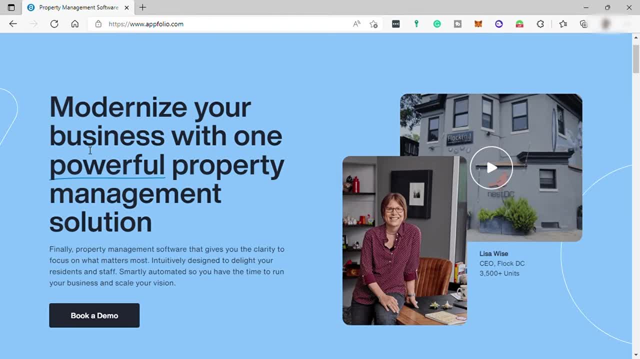 Upfolio Property Manager is a cloud-based property management software that allows multi-family and single-family commercial student housing homeowners and condo association and a mixed portfolio of property managers to market, manage and grow their business. Upfolio includes complete accounting and property management functionality. 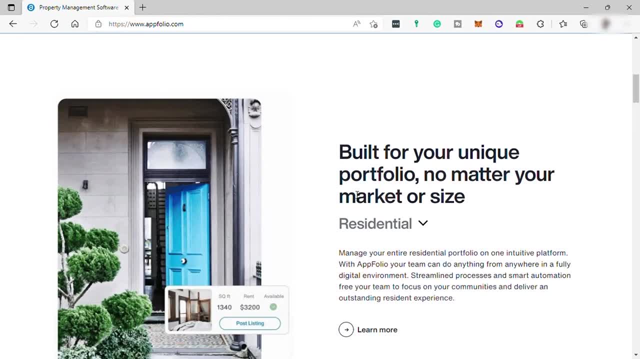 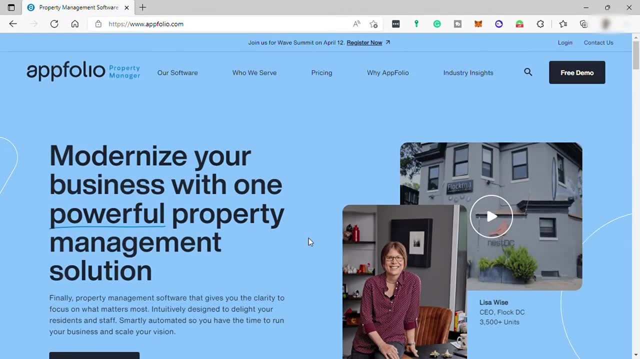 including the ability to provide instant access to reports and statements, post and market vacancies, apply and lease online. screen residents, streamline rent collection and mobile inspections. Features highlighted on this software are: self-service online owner and renter portals, online applications and leases, online payments. built-in screening maintenance request. 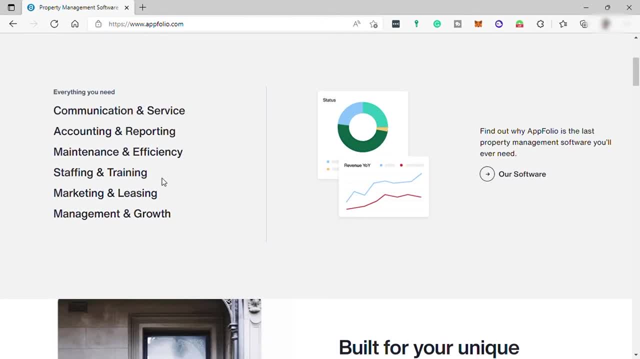 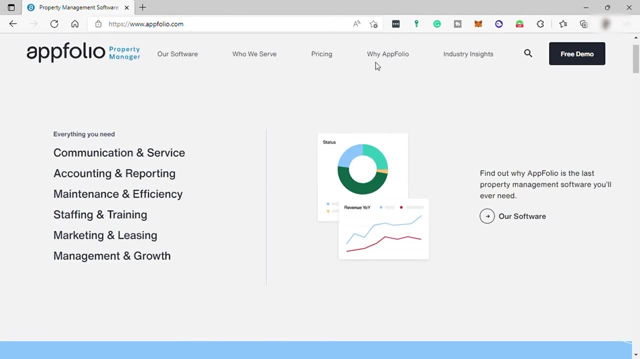 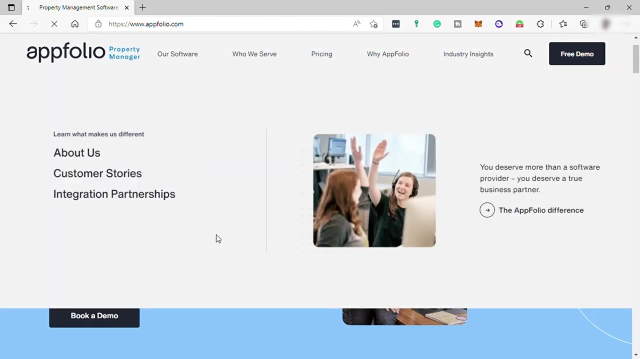 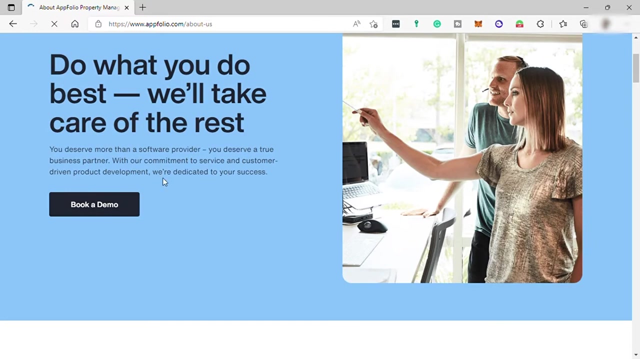 mobile inspections, book text messaging, accounting and reporting and a seamless mobile app. experience Also includes property listing management, cash flow management, landlord insurance, trucking, automatic billing, posting, paperless work order generation, report, customization and more. Also, the most important is that all Upfolio customers receive access to training and 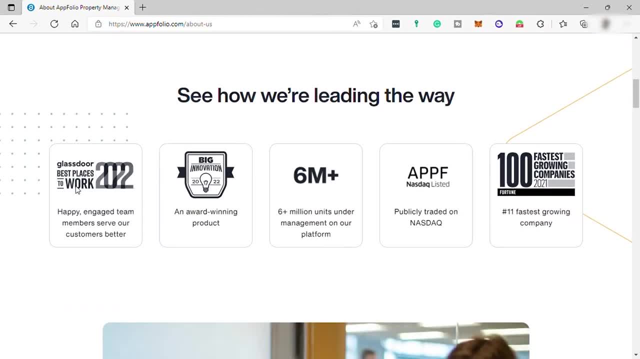 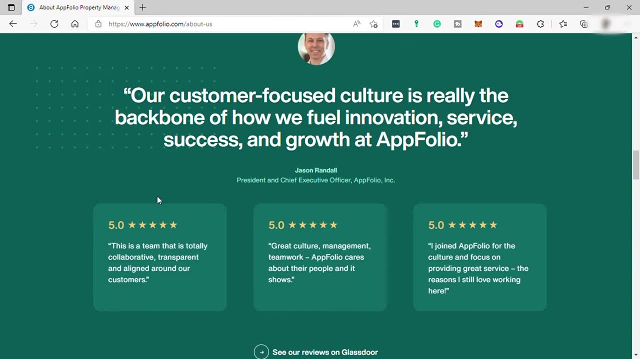 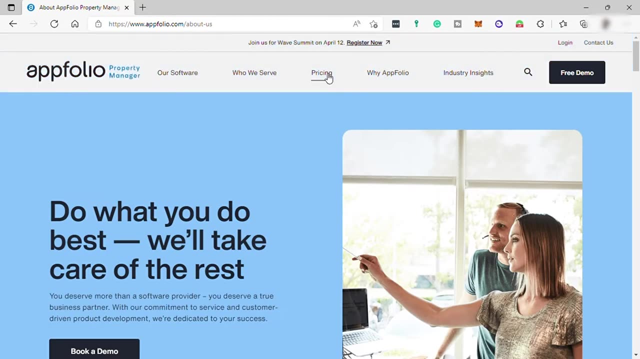 health resources, as well as an award-winning support team. Finally, a property management software that gives you the clarity to focus on what matters. So before we start, let's first check its pricing plan. So going to pricing up here and you'll see. 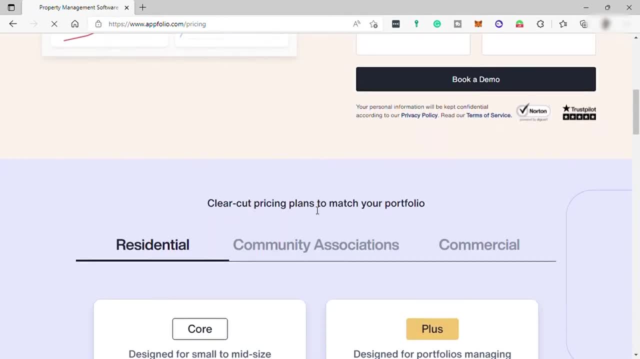 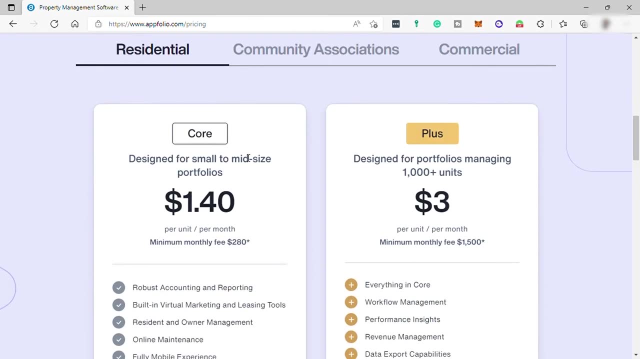 they have three different categories and just choose what's perfect for your business. They have first for residential and the residential. they have two different plans. First is the core plan, designed for small to mid-size portfolios for $1.40 per unit per month. And the minimum monthly fee is $1.40 per month. So that's the minimum monthly fee, So that's the is $280 per month. You can have robust accounting and reporting built-in. virtual marketing and leasing tools, resident and owner management, online maintenance- fully mobile experience. 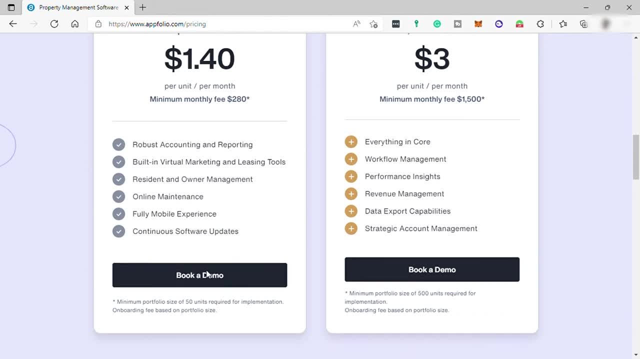 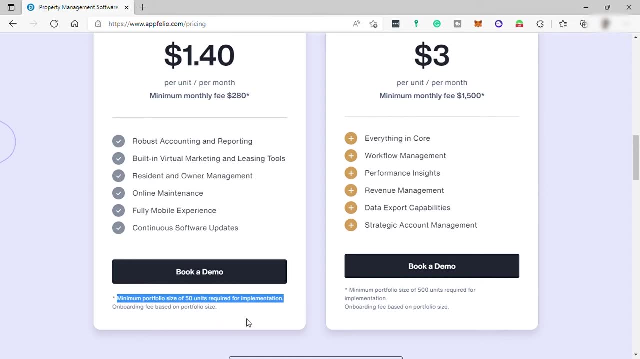 and continuous software updates, And it's minimum portfolio size of 50 units required for implementation, So you need to have 50 units to avail this plan. The second is the plus plan, designed for portfolio size, So you need to have 50 units to avail this plan. And the second is the 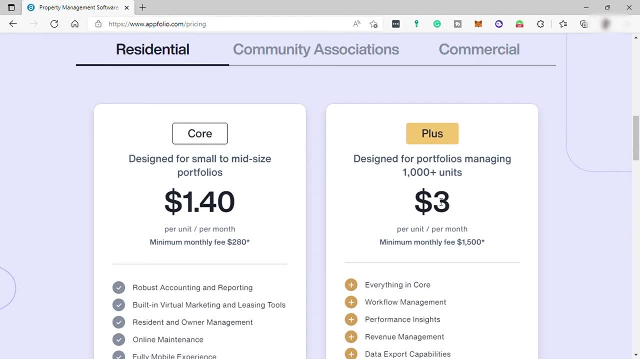 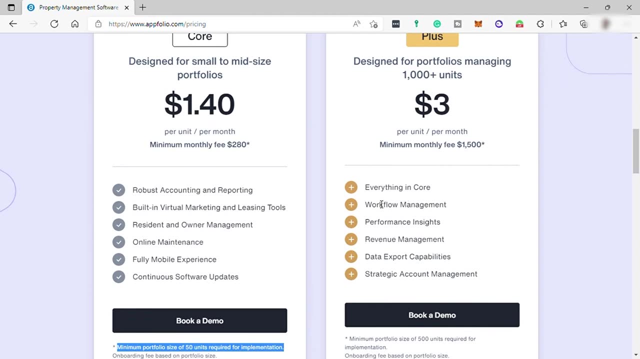 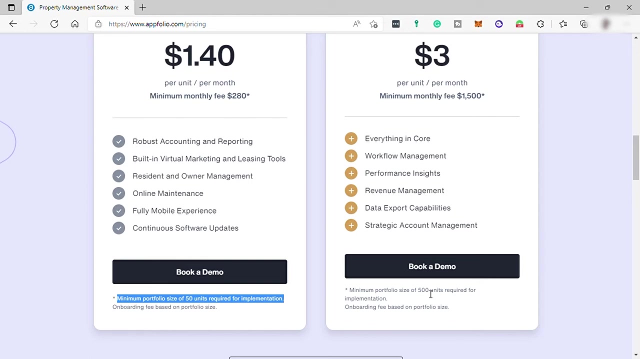 managing 1,000 plus units for $3 per unit per month. It includes everything in core plan plus workflow management, performance insight, revenue management, data export capabilities, strategic accounting management and its minimum portfolio size of 500 units required for implementation. So the next category or business is community association. 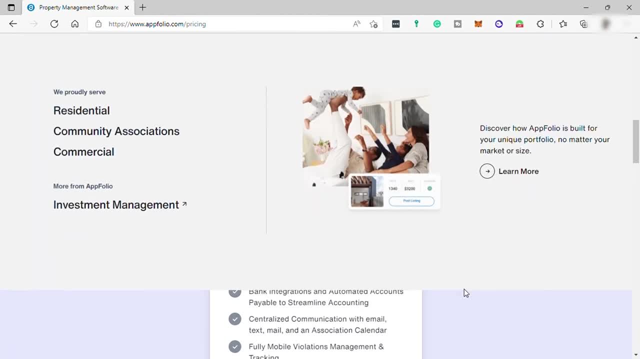 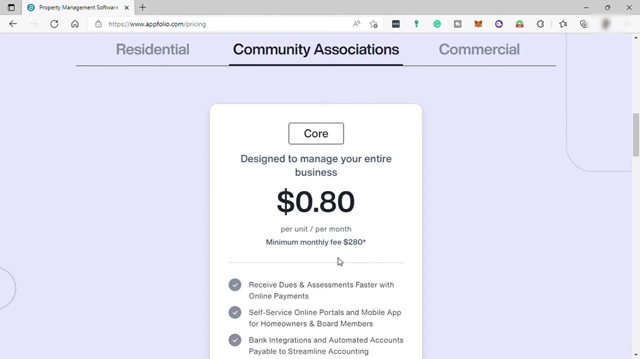 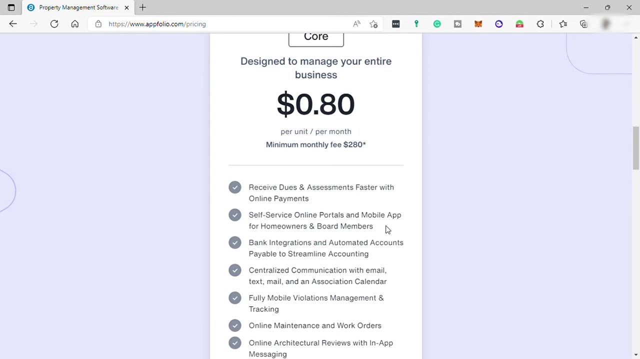 In this category there is only one plan, which is the core plan, designed to manage your entire business for $0.80 per user per month, And you will be receiving dues and assistance faster with online payments, self-service online portals and mobile app for homeowners and board members. 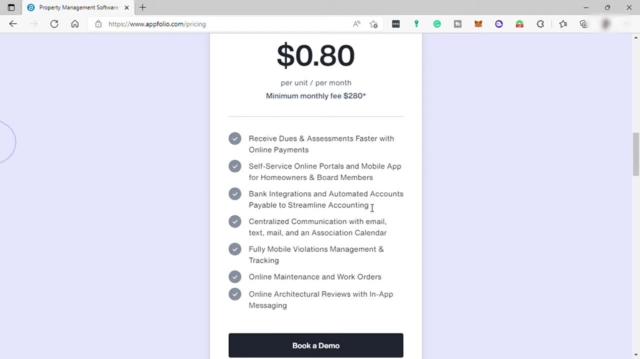 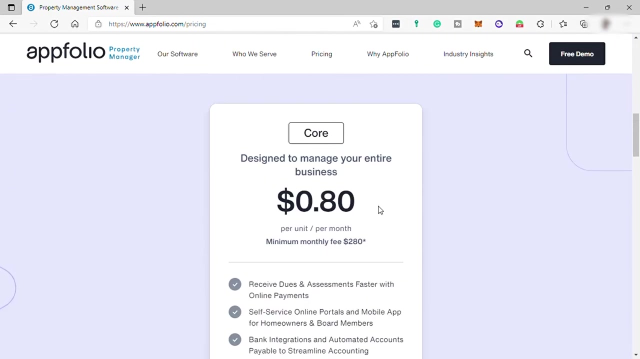 bank integration and automated accounts payable to streamline accounting. centralized communication with email, text mail and an association calendar. fully mobile violation management and tracking, online maintenance and work orders, online architectural reviews and in-app messaging. The last one is for commercial businesses. They have two different plans here. First is the core. 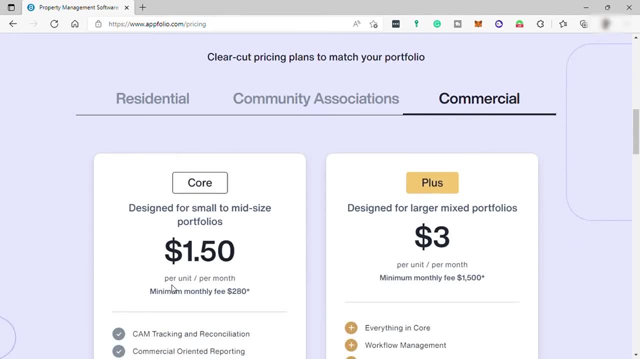 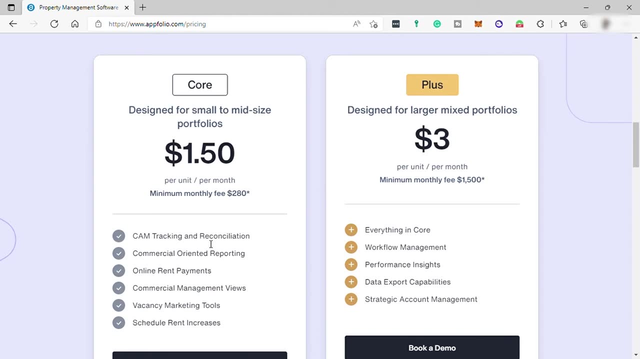 plan for $1.50.. And these are the features covered in this plan: Calm or CAM, tracking and reconciliation, commercial-oriented reporting- and the last one is the core plan for commercial businesses And the last one is for commercial businesses, And these are the features covered in this plan. 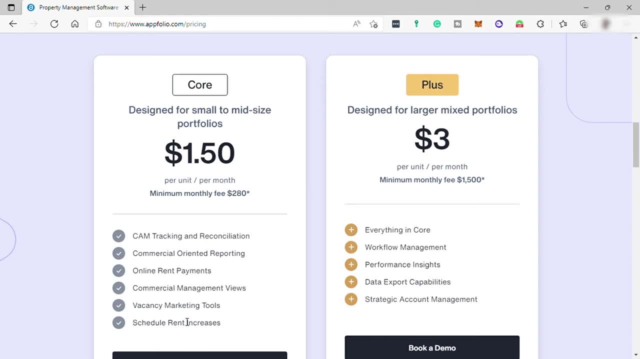 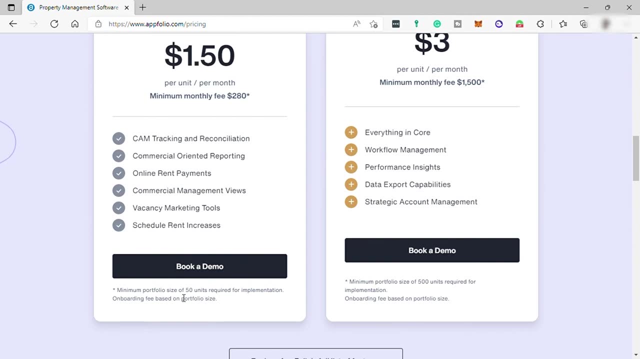 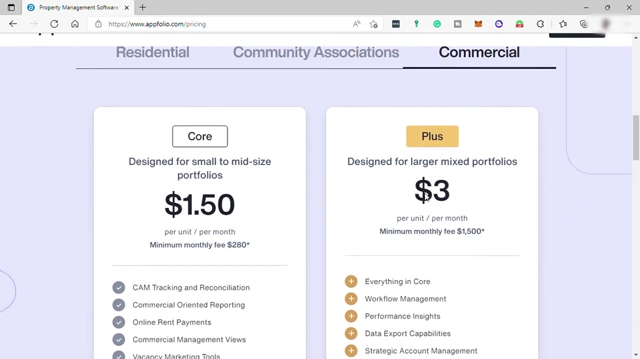 Online rent payments, commercial management views, vacancy marketing tools and schedule. rent increased Also minimum portfolio size of 50 units required for implementation for this plan And the next one is the plus plan designed for larger mixed portfolios, for $3 per unit per user. 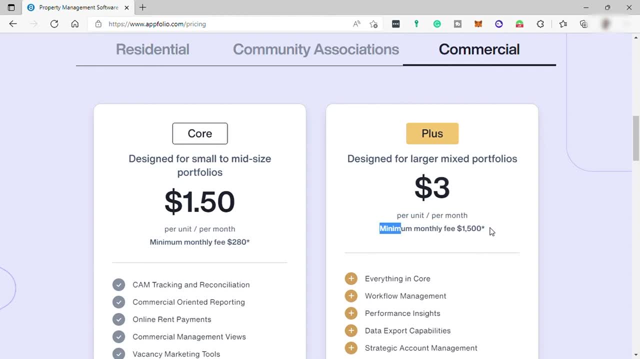 and minimum monthly fee of $1,500 per month. And, by the way, for the core plan, the minimum monthly fee is $1,500 per month And the next one is the plus plan, designed for larger mixed portfolios, for $3 per unit per user and the minimum monthly fee of 1,500 per month. 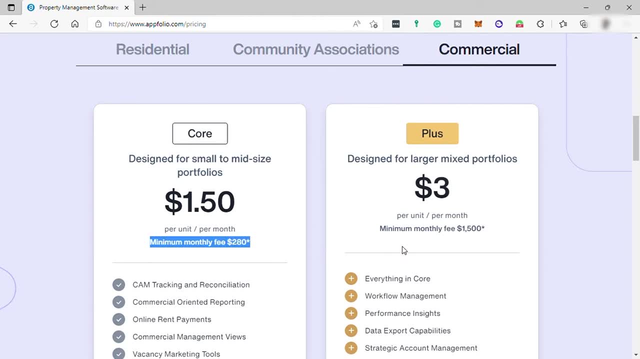 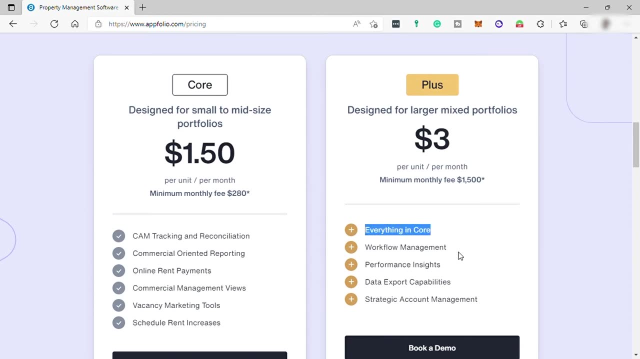 And the next one is the plus plan, designed for larger mixed portfolios, for $3 per unit per user and the minimum monthly fee is $280.. So, going back to the plus plan, you will have this feature. everything in core are included, plus workflow management, performance insights, data export capabilities, strategic account. 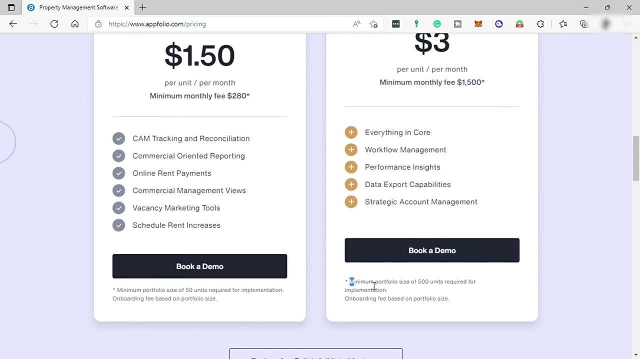 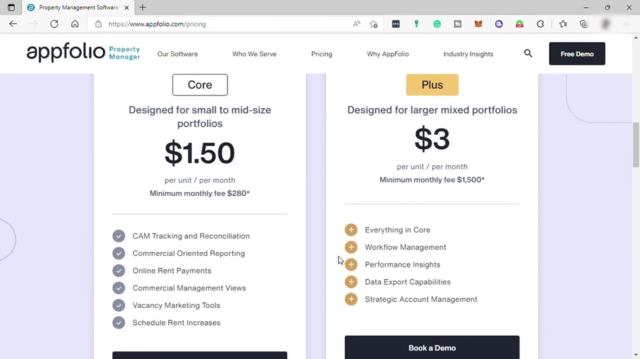 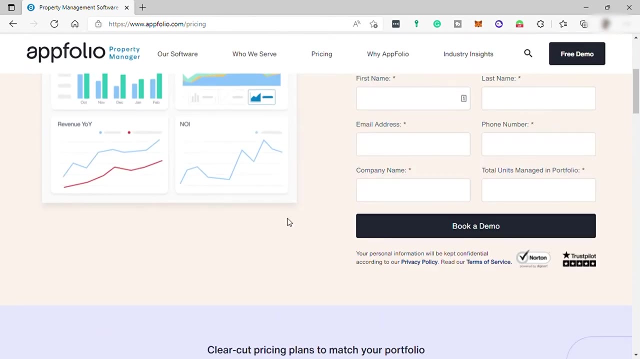 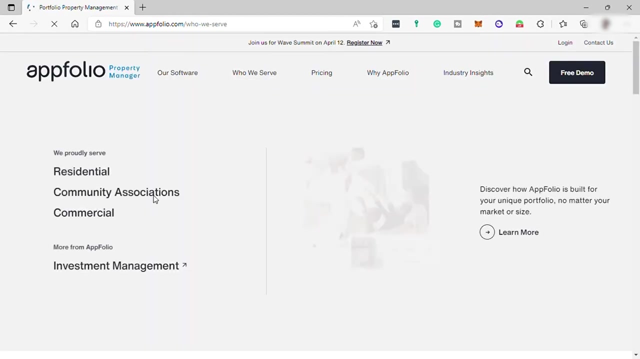 management and the minimum portfolio size of 500 units required for implementation in this plan. So these are the different pricing plan of Upfolio in different portfolios. So to find out or learn more about these three categories, you can check here. So let's just go to who we serve And here you can see all the information here about these. 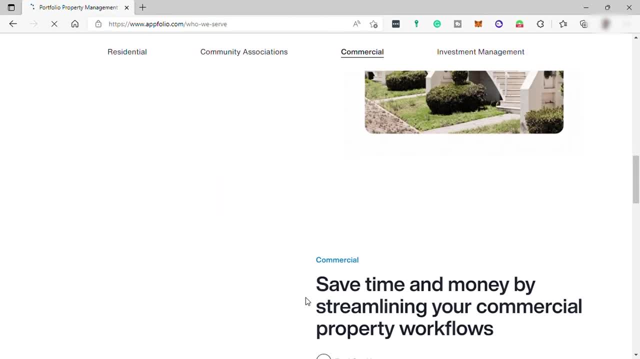 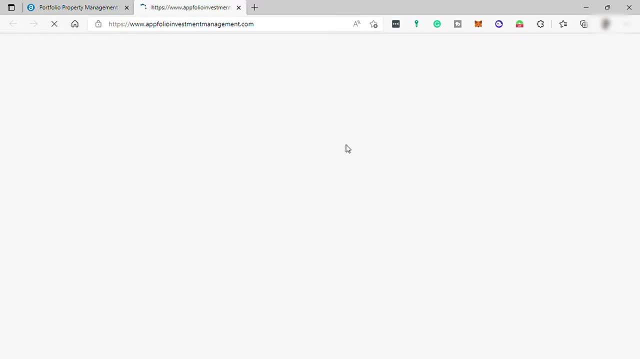 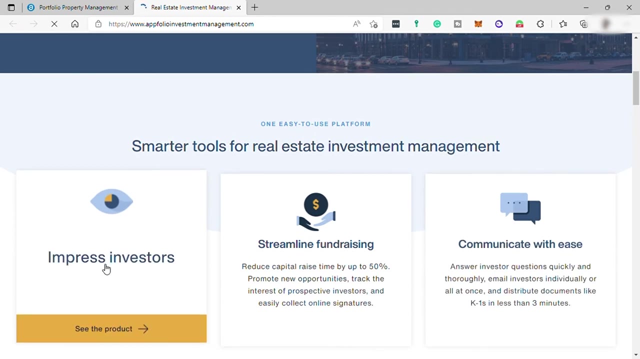 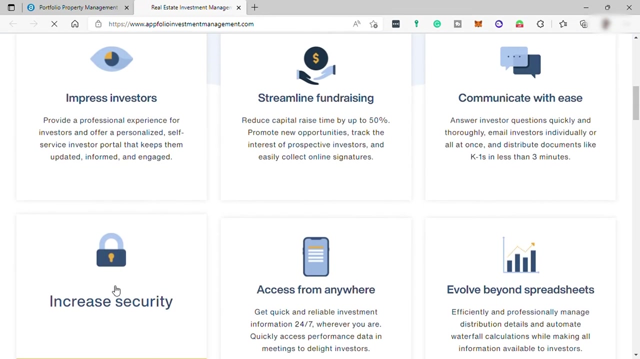 three different categories. You will see here their differences- And they have also investment management. So this tool is your complete real estate investment management solution tool And this is a smarter tool for real estate investment management to impress your investor. streamline fundraising, communicate with your investor with ease, increase security. 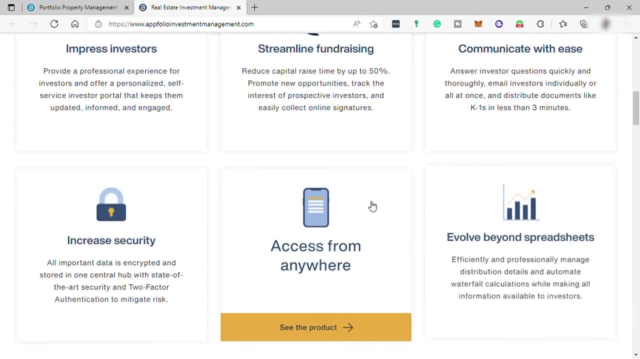 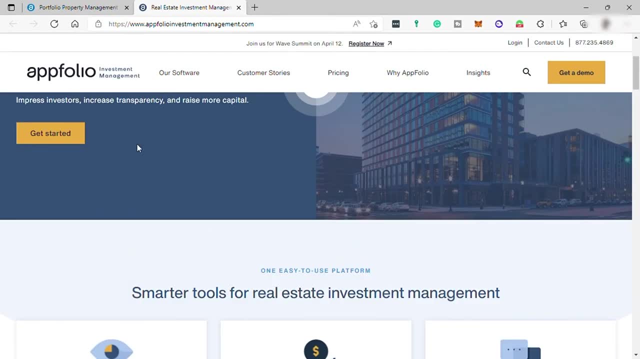 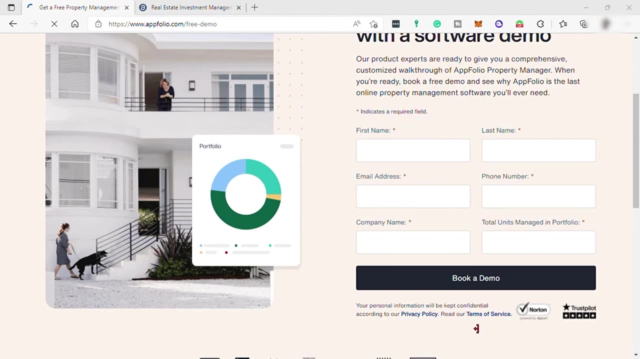 and access this tool anywhere and anytime you like and more. To create an account here to start your business with Upfolio, you need to first book a demo. So click here on free demo and then just fill out this form And then, once you're done, click, book a demo Once you request a demo. 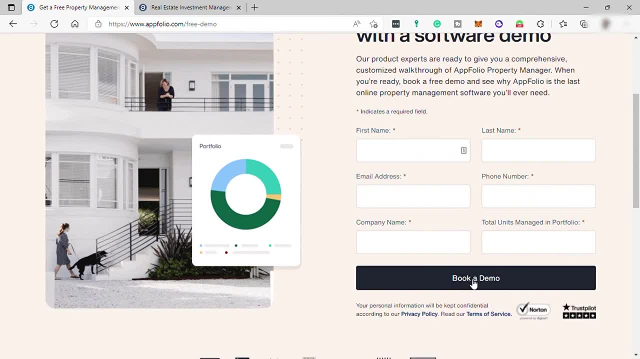 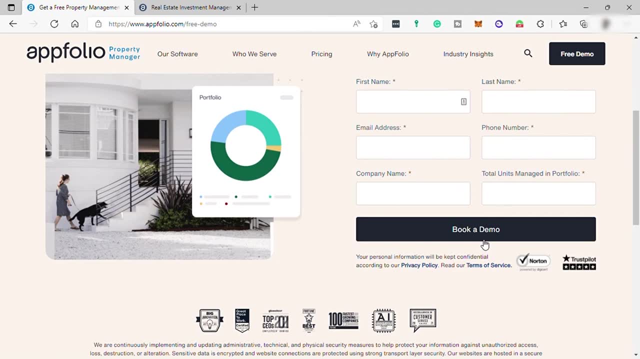 a member of their team will reach out to you to serve as your first point of contact and set up a quick introductory call to learn more about your portfolio, your properties and business structure. After that, they will dive deeper into your specific needs and they will match you up with. 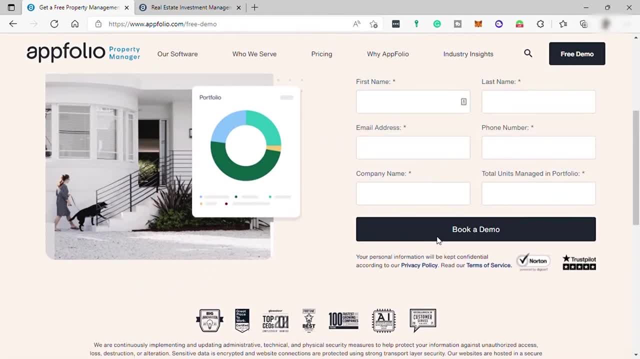 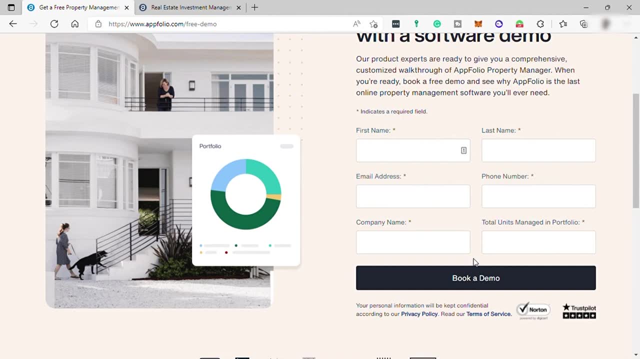 a specific specialist with the right expertise who will construct, plan and schedule a customized demo for your business so that they can help you along the way in your business. So this is a great way to start your business here in Upfolio. So you need all of this before you can start. 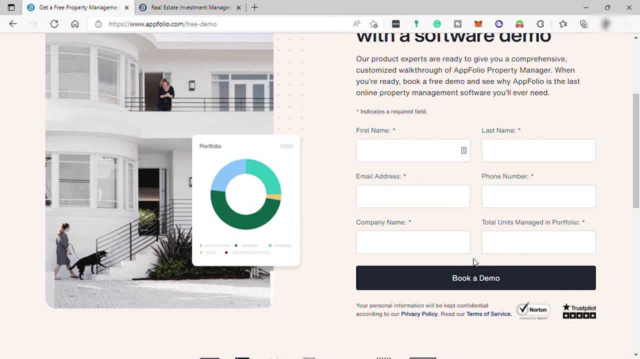 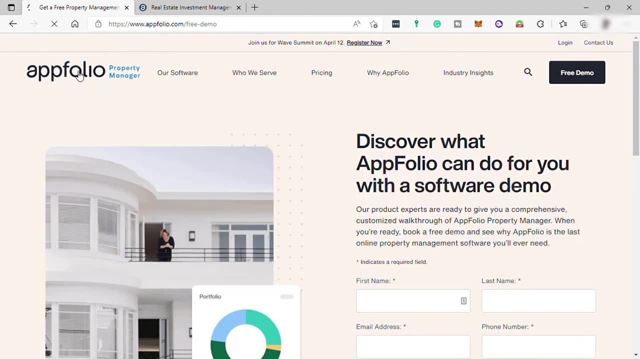 creating an account and use their software. So you need to first get a demo, talk to them and have communication with their specialists before you can have business with them. This software is perfect for those business people who have property or real estate business. 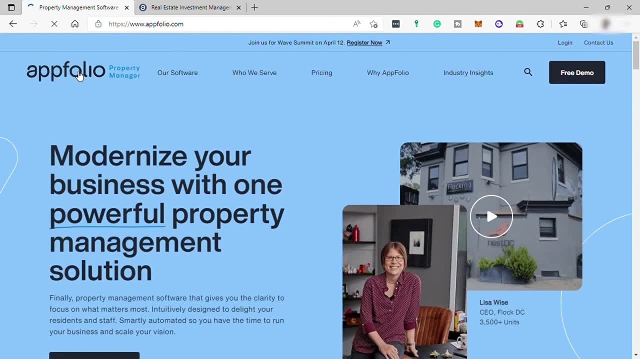 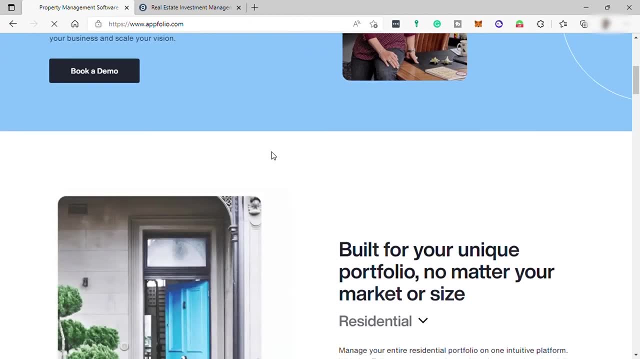 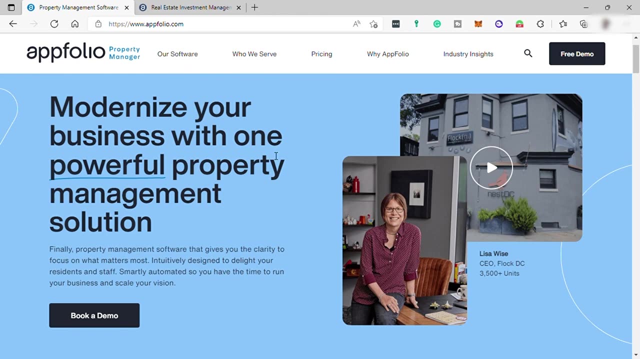 Upfolio is very secure software for your business and also they receive different awards in previous years. That includes Upfolio WINS, the 2020 Artificial Intelligence Excellence Award. The Artificial Intelligence Excellence Awards are hosted by the Business Intelligence Group, which recognizes businesses products.